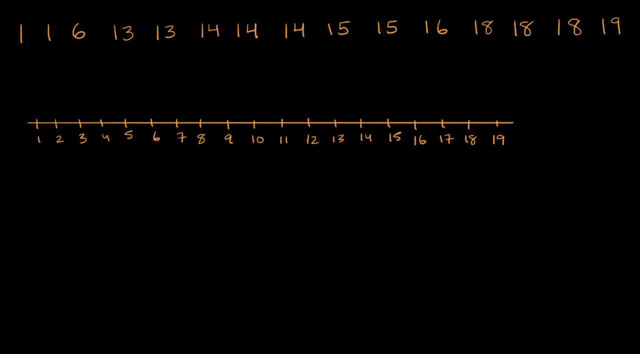 from one to 19.. And let's see, we have two ones. So I could say that's one one and then two ones. We have one six. so let's put that six there We have got 13,. or we have two 13s. 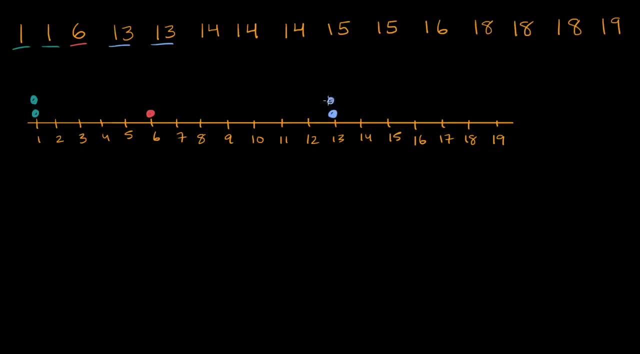 So we're gonna go up here One 13 and two 13s. Let's see we have three 14s, So 14,, 14, and 14.. We have a couple of 15s: 15,, 15.. 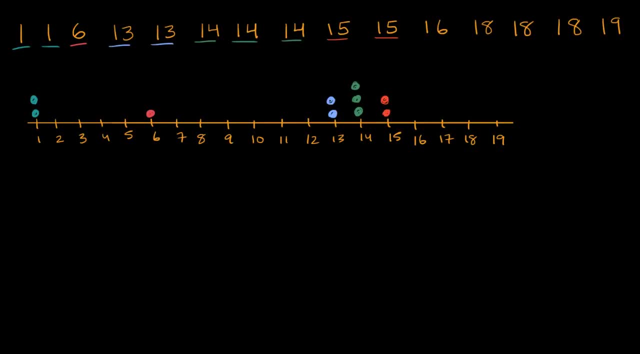 So 15,, 15.. We have one, 16. So that's our 16. there We have three 18s. One, two, three. So one, two and then three, And then we have a 19.. 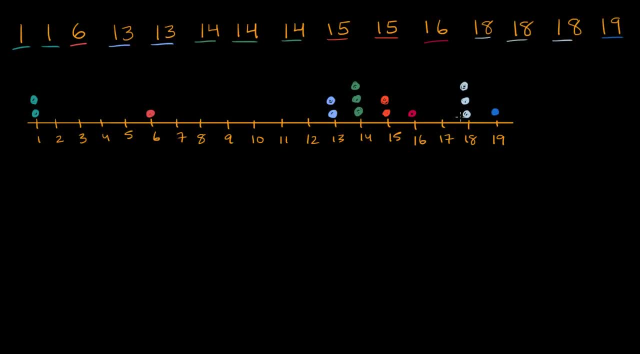 And then we have a 19.. So when you look visually at the distribution of numbers, it looks like the meat of the distribution, so to speak, is in this area, right over here, And so some people might say, okay, we have three outliers, these two ones, 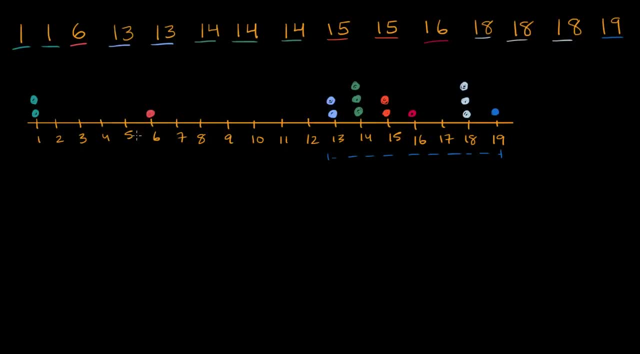 and the six, Some people might say: well, the six is kinda close enough. Maybe only these two ones are outliers, And those would actually be both reasonable things to say. Now, to get on the same page statisticians, we'll use a rule sometimes. 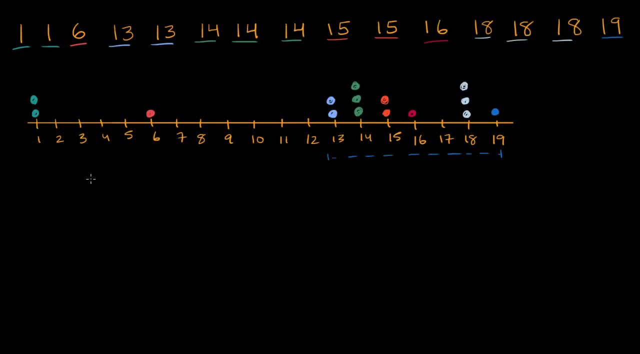 We say: well, anything that is more than one and a half times the interquartile range from below Q1 or above Q3, well, those are going to be outliers. Well, what am I talking about? Well, let's- actually let's- figure out the median. 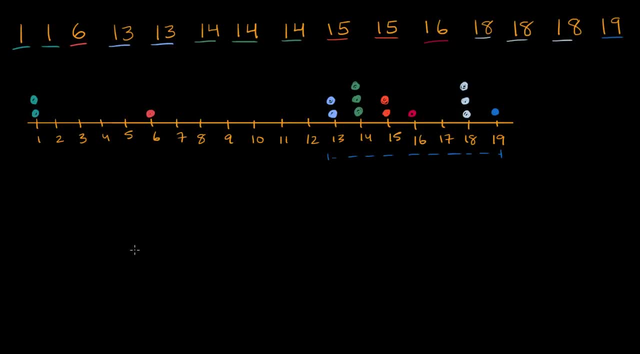 Let's figure out the median Q1 and Q3 here, Then we can figure out the interquartile range and then we can figure out by that definition what is going to be an outlier And if that all made sense to you so far. 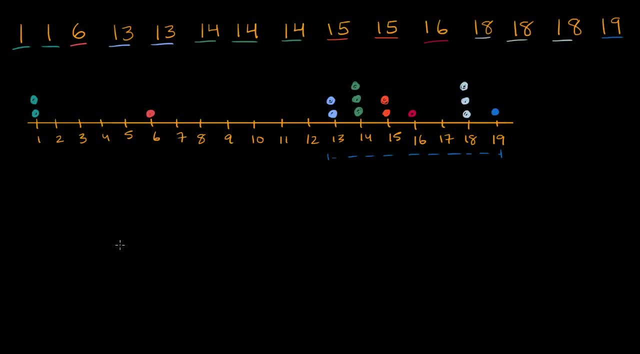 I encourage you to pause this video and try to work through it on your own, or I'll do it for you right now. All right, so what's the median here? Well, the median's the middle number. We have 15 numbers, so the middle number 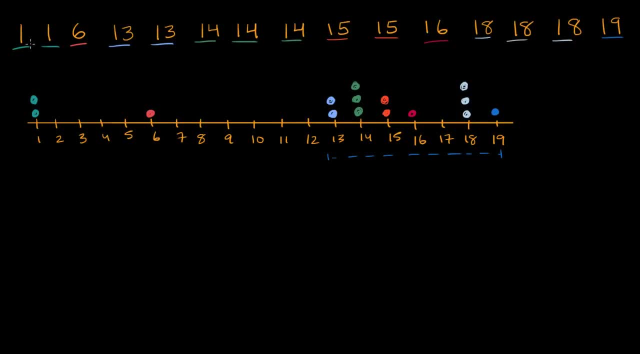 is going to be. whatever number has seven on either side, so that's gonna be the eighth number. One, two, three, four, five, six, seven, eight, nine, 10,, 10, seven, is that right? 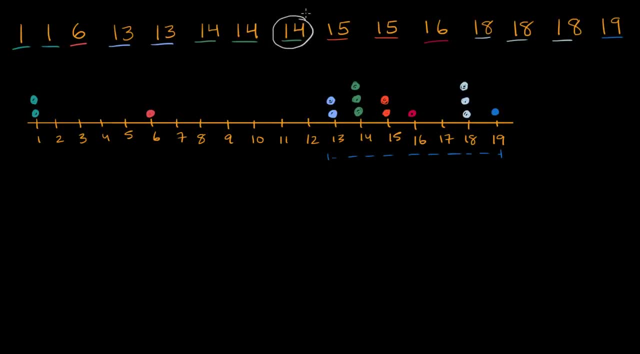 Yep six, seven. so that's the median. And you have one, two, three, four, five, six, seven numbers on the right side too. so that is the median, sometimes called Q2.. That is our median. 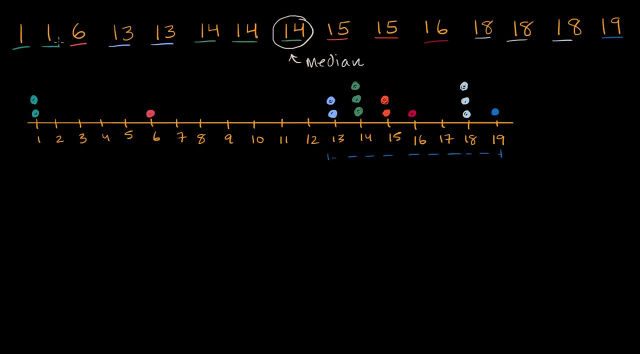 Now, what is Q1?? Well, Q1 is going to be the middle of this first group. This first group has seven numbers in it, and so the middle is going to be the fourth number. It has three and three, three to the left. 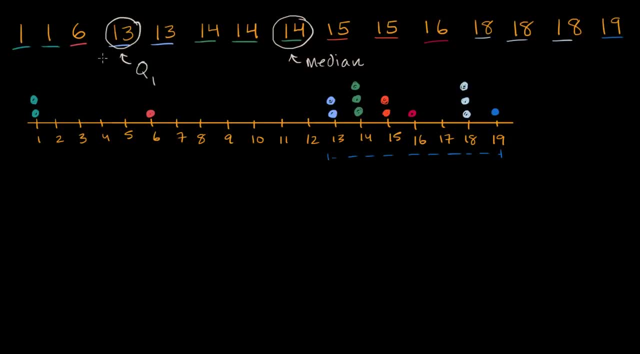 three to the right, So that is Q1. And then Q3 is going to be the middle of this upper group. Well, that also has seven numbers in it, so the middle is going to be right over there. It has three on either side. 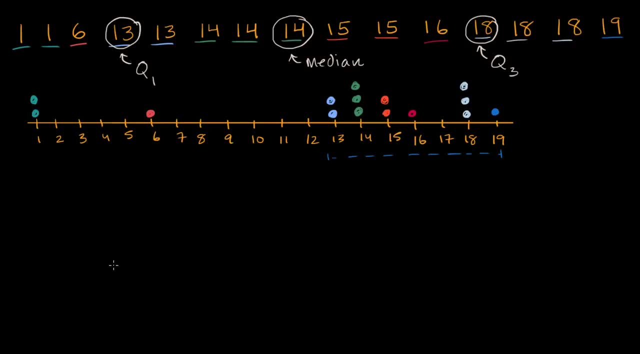 So that is Q3.. Now what is the interquartile range going to be? Interquartile range is going to be equal to Q3 minus Q1. The difference between 18 and 13. Between 18 and 13.. 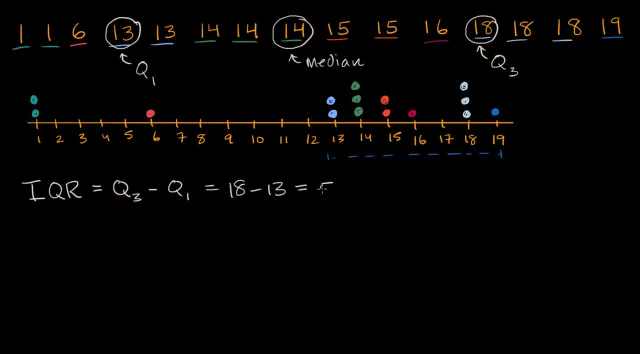 Well, that is going to be 18 minus 13,, which is equal to five. Now to figure out outliers. well, outliers are going to be anything that is below. So outliers outliers are going to be less than our Q1 minus 1.5 times our interquartile range. 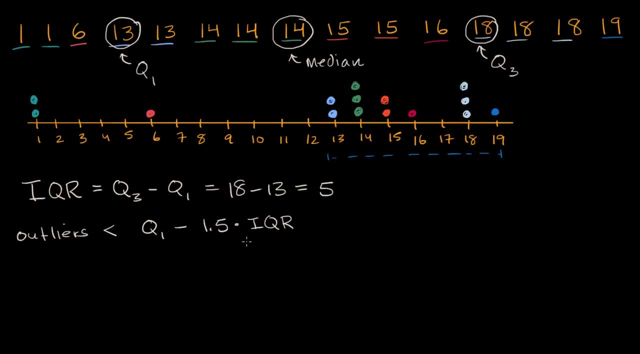 And this once again, this isn't some rule of the universe. This is something that statisticians have kind of said. well, if we want to have a better definition for outliers, let's just agree that it's something that's more than 1.5 times the interquartile range below Q1,. 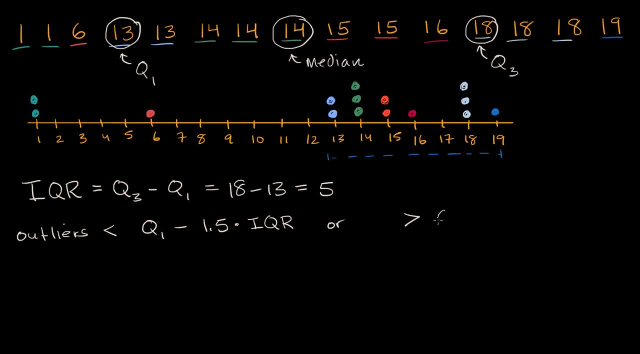 or an outlier, could be greater than Q3 plus 1.5 times the interquartile range. interquartile range- And once again this is somewhat you know- people just decided it felt right. One could argue it should be 1.6,. 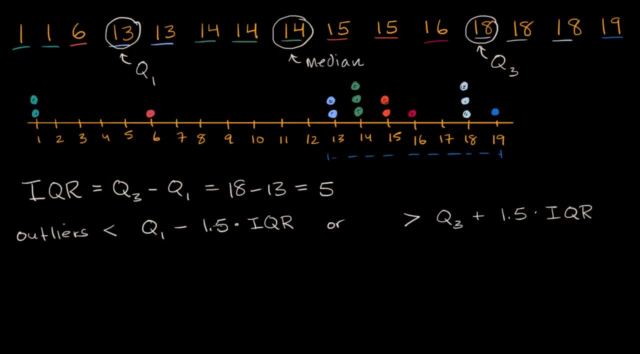 or one could argue it should be one or two or whatever, but this is what people have tended to agree on. So let's think about what these numbers are. Q1, we already know. so this is going to be 13 minus 1.5 times our interquartile range. 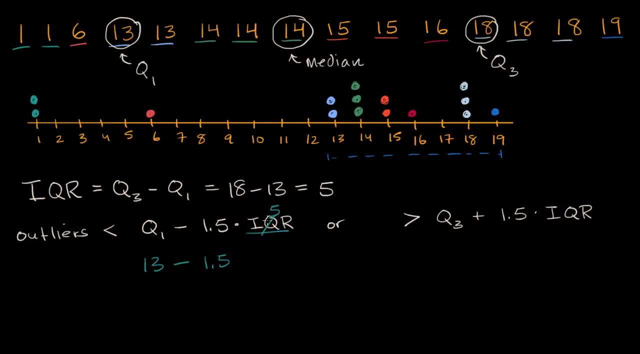 Our interquartile range here is five, So it's 1.5 times five, which is 7.5.. So this is 7.5.. 13 minus 7.5 is what? 13 minus seven is six, and then you subtract another .5. 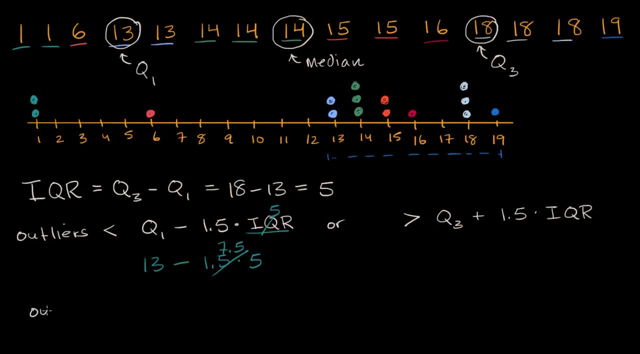 is 5.5, so we have outliers, outliers. Outliers would be less than 5.5, or Q3 is 18, this is once again 7.5.. 18 plus 7.5 is 25.5,. 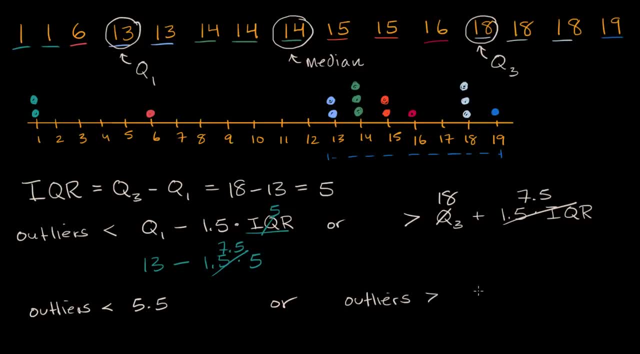 or outliers: outliers greater than 25,, 25.5.. So based on this, we have a kind of a numerical definition for what's an outlier. We're not just subjectively saying, oh, this feels right or that feels right. 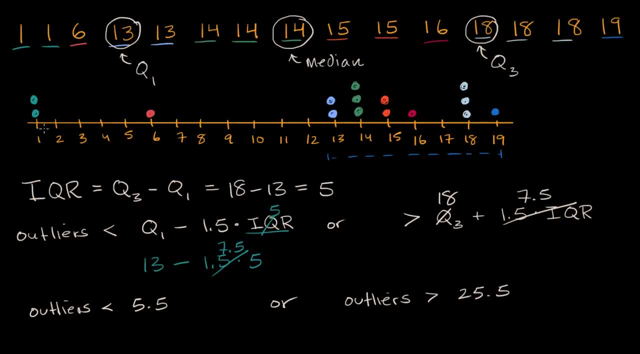 And based on this, we only have two outliers, that only these two ones are less than 5.5.. Only these two ones are less than 5.5.. This is the cutoff right over here. So this dot just happened to make it. 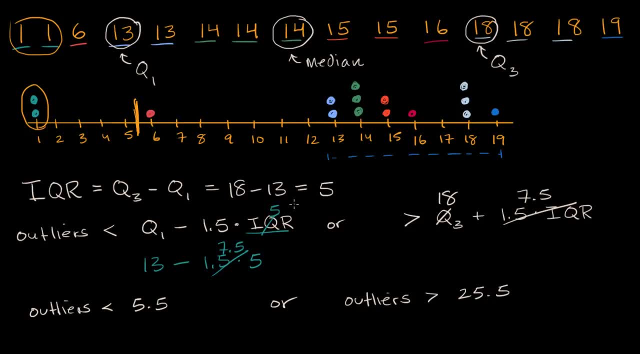 and we don't have any outliers on the high side. Now, another thing to think about is drawing box and whiskers plots based on Q1, our median, our range, all the range of numbers, and you can do it either, taking in consideration 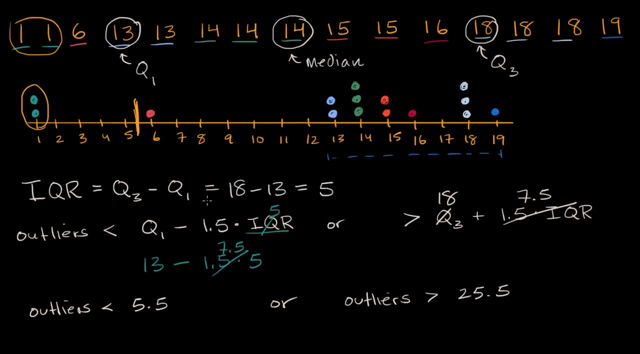 your outliers or not taking into consideration your outliers. So there's a couple of ways that we can do it. So let me actually clear, let me clear all of this. We've figured out all of this stuff, So let me clear all of that out. 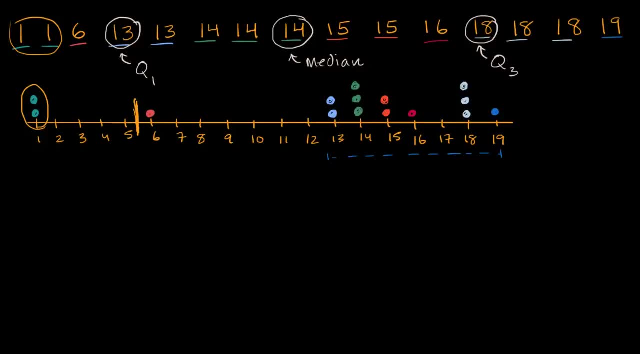 And let's actually draw a box and whiskers plot, So I'll put another. actually let me do two here. That's one, and then let me put another one down there, And this is another. Now, if we were to just draw a classic box, 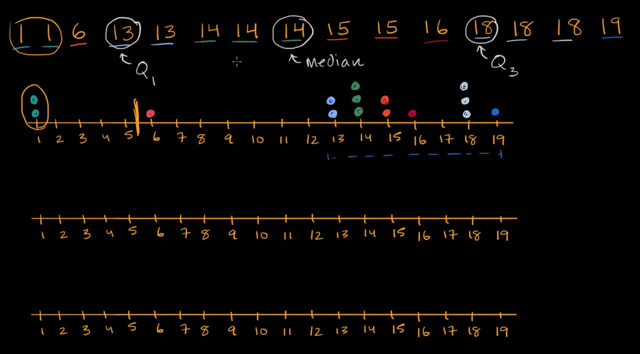 and whiskers plot. here we would say: all right, our median's at 14, and actually I'll do it both ways: Our median's at 14,, Q1's at 13,, Q3 is at 18, so that's the box part. 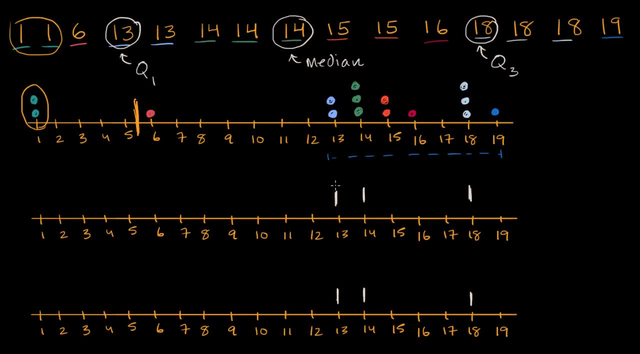 And let me draw that as an actual, let me actually draw that as a box. So my best attempt, There you go. that's the box And this is also a box. So far, I'm doing the exact same thing. Now, if we don't want to consider outliers,